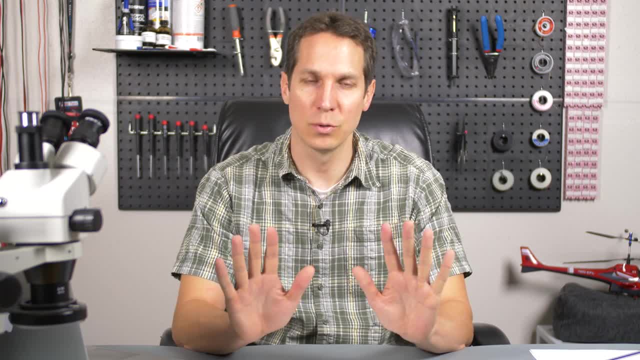 base 10.. And that is because we have 10 fingers. At least that's what we think And it makes sense to me. So we can say: hey, I want 10 things, Oh, no, I want 20 things, I want 30 things. 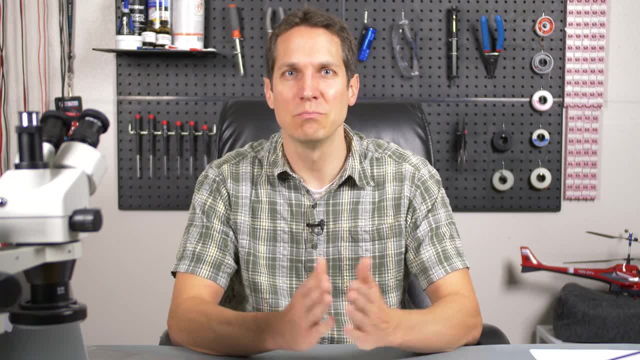 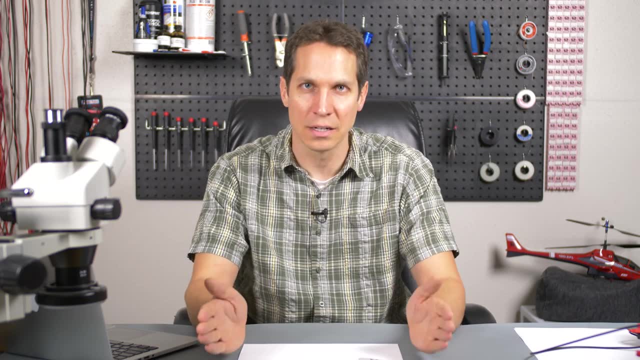 something like that, And so that is how we count. No reason to mess with it, Except if you're going to be working with embedded systems, computers, anything like that. everything there is in binary, And then, for reasons that you may or may not understand, they're also in hexadecimal, So 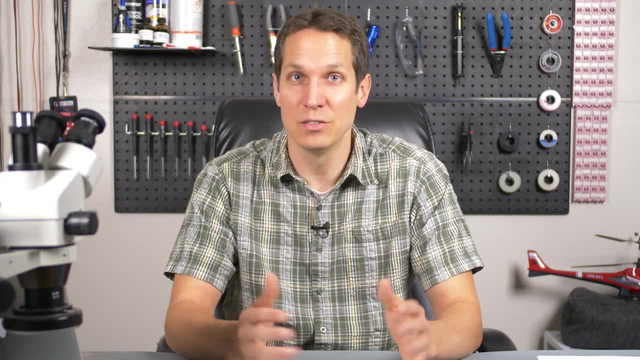 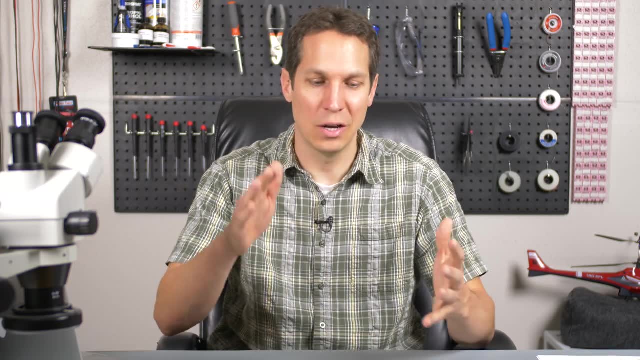 we're going to go over basically why base 10 is the way it is, decimal, the way we count currently, what base 2 is, what hexadecimal is, why we use it, And then you're going to understand not only how these all work together but also how to. 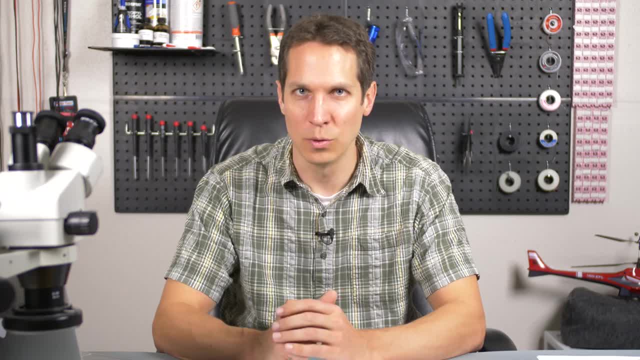 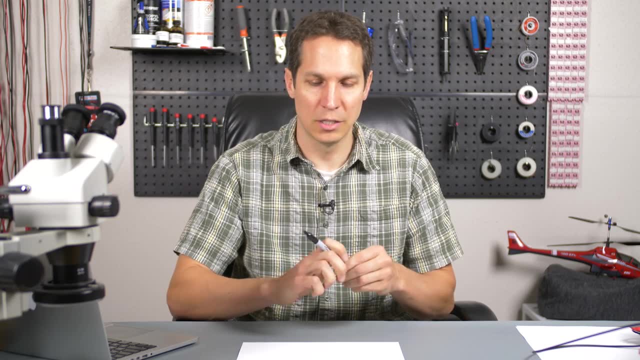 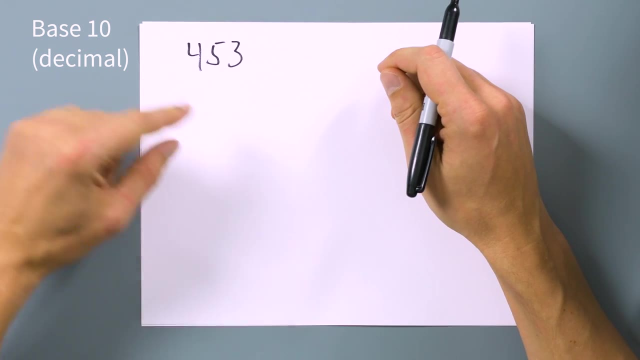 convert from one to the other, and why hexadecimal is so darn cool. So first things first. let's talk about base 10 or decimal. So let's take a number. I'm going to randomly come up with a number. let's say 453.. So 453.. Now the interesting thing is, if you look at it, the numbers that make up 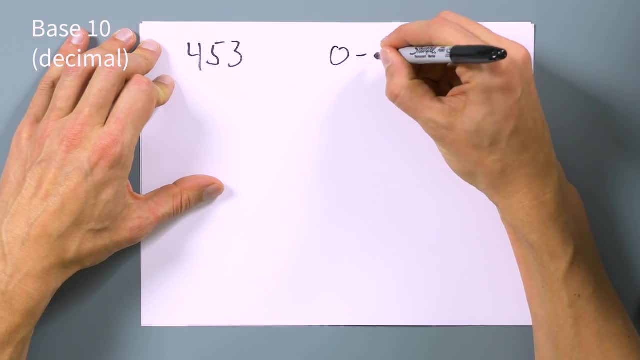 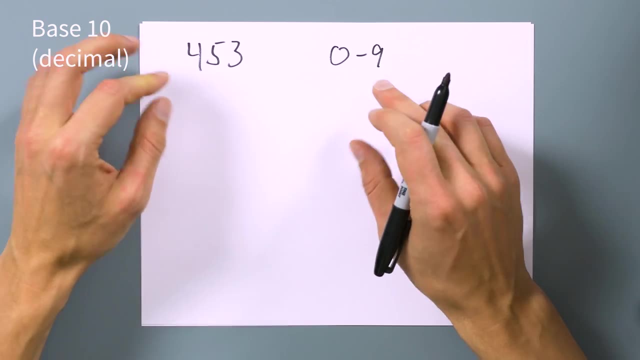 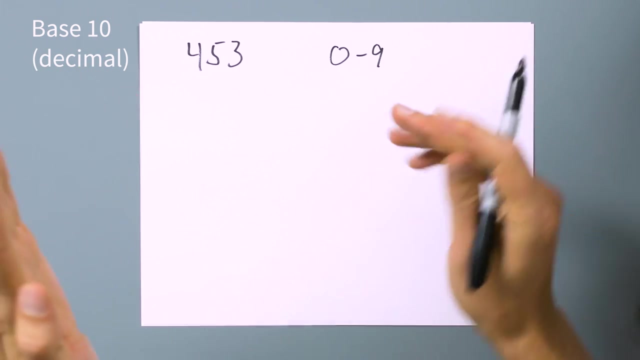 our numbers actually only range from zero to nine, So there's only 10, 10 actual numbers. Once we get up to nine, instead of coming up with another number, we'll just call it Bob. for no reason it's zero to Bob, we go one zero. So when you're looking at 453, right here, 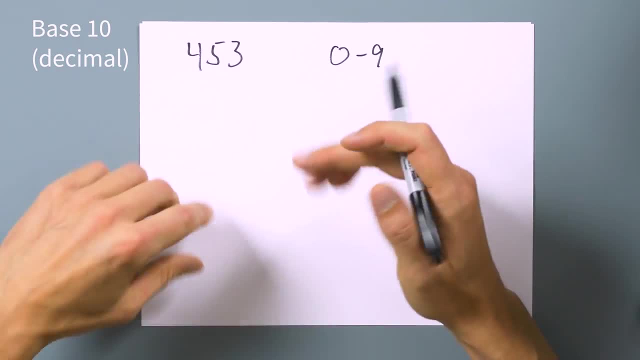 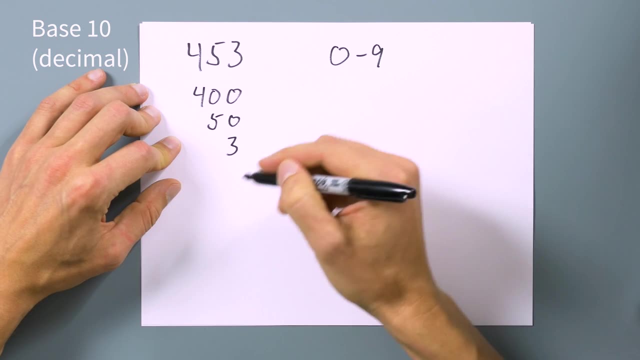 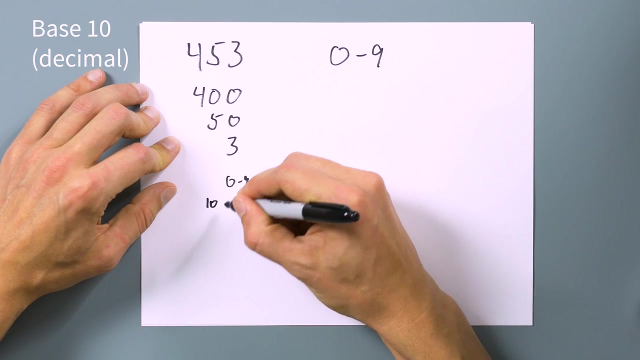 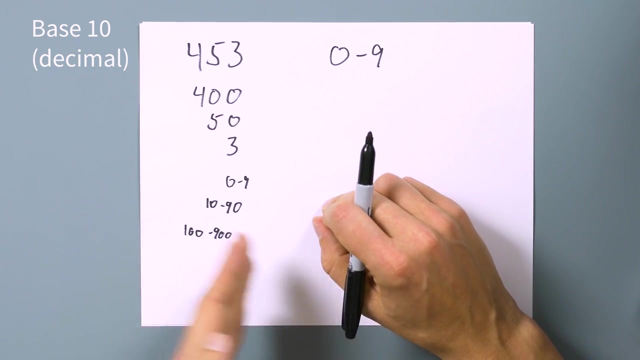 you're not actually looking at a single number. you're looking at 400 plus 50, plus three, and that comes out to 453.. And so, basically, what you have here is zero to nine. you have here 100, to 900. And then you just change each one as you need to. Now, the way this is broken up is you: 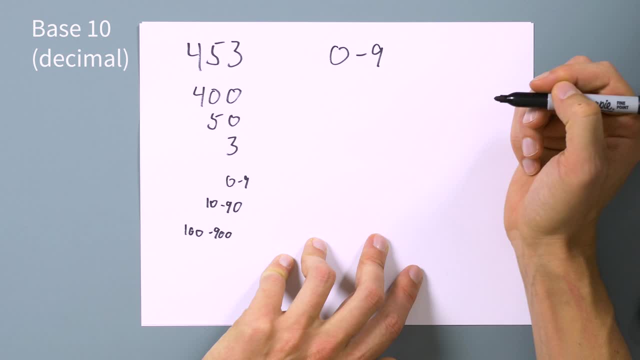 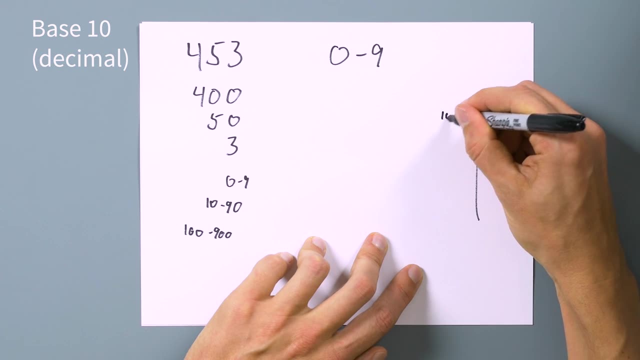 basically look at it- and you can look at it top down to make it make more sense- And you just want to say, okay, zero to nine. And then what am I doing? 10 to 90? 100 to 900.. And then this keeps. 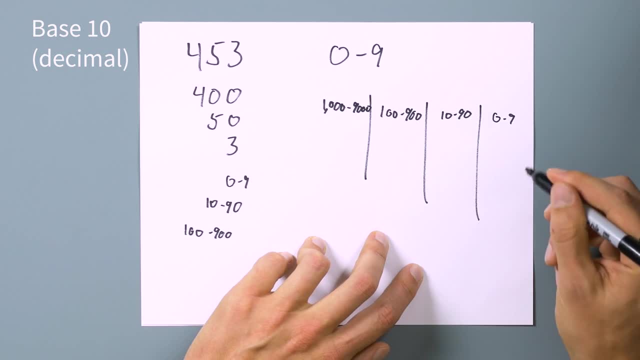 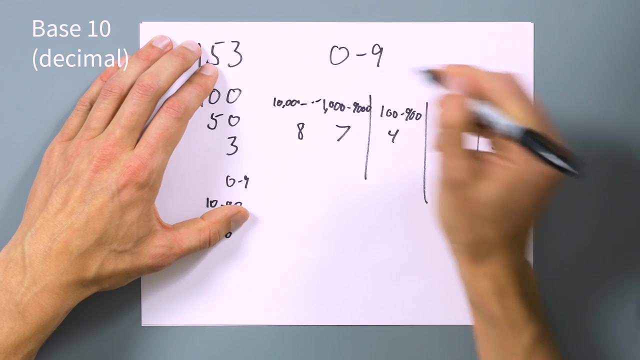 on going 1000 to 9000. And then you just change each one as you need to, And then you just change. You just throw in whatever numbers you want there to make what you want. So now I have 7453, Hey, I want 87,000, and doing that's how it goes. 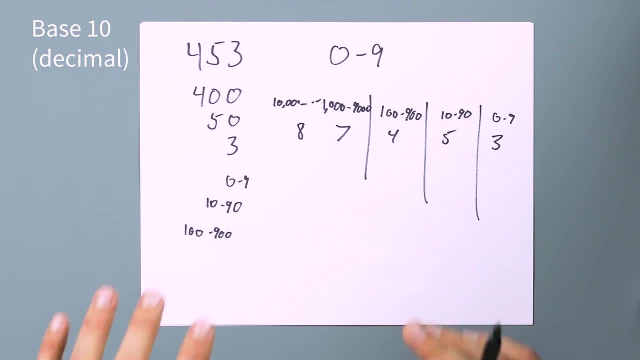 So that is generally how our base 10 works. Now, to make this more generic, let's do this as: 10 to the zero, 10 to the one, 10 to the two, 10 to the three- wow, that 10 got really ugly- and 10 to the four. 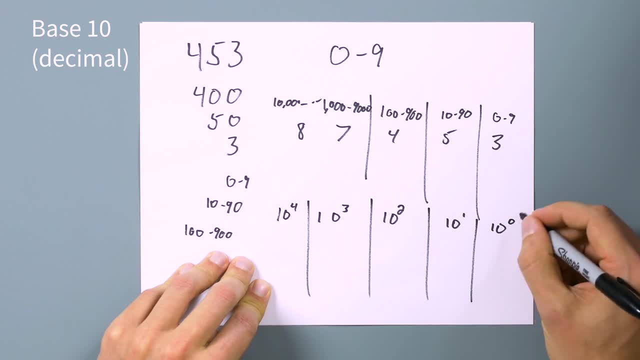 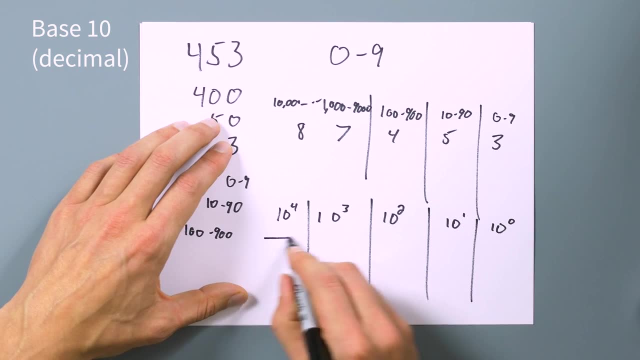 Now you'll notice that's the same: 10 to the zero, anything to the zero is one. So that multiplier is then multiplied by whatever number you have underneath. So that's three times one, That's five, That's five times 10.. 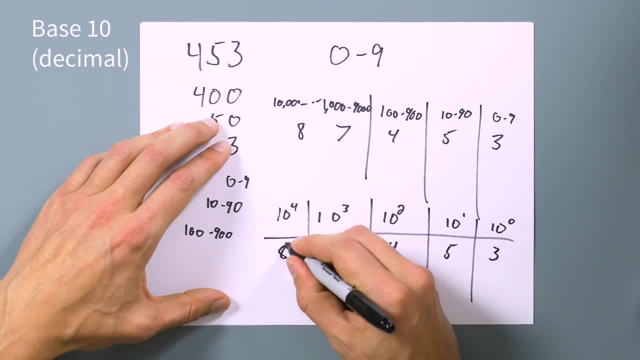 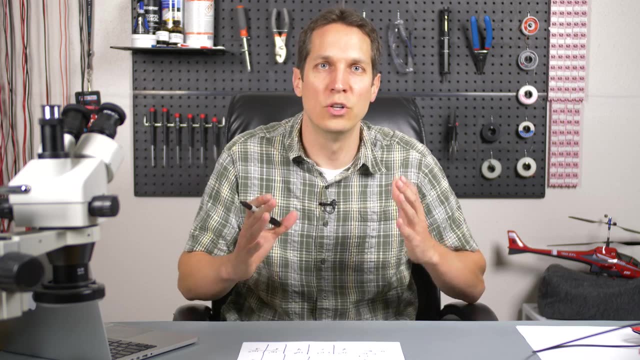 That's four times 100. That's seven times 1000, eight times 10,000. And that's how you get 87,453.. So that is how our numbering system works. If you understand this, it's going to make understanding binary way easier. 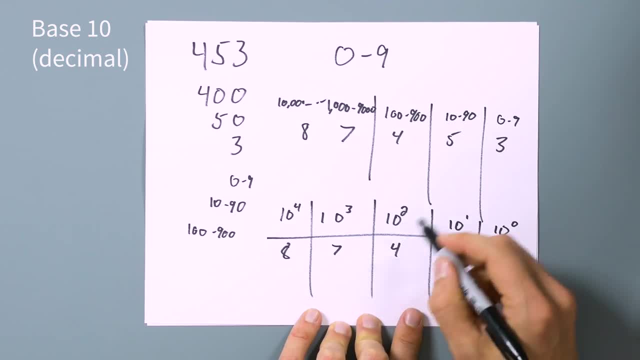 So this is base 10.. And so that is 10 to the zero, 10 to the one, 10 to the two, 10 to three, which goes on for infinity. 10 to the five. It's always incremented by one, but it just goes on forever. 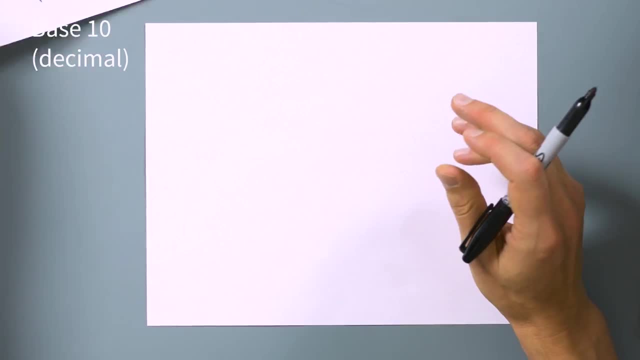 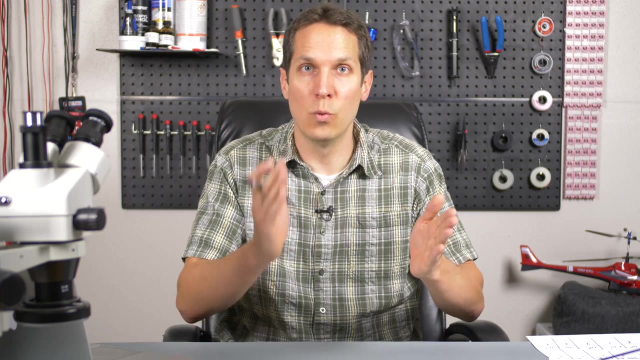 Now, if we're going to do, If we're going to do binary, which is base two, it's going to be slightly different. Now, the reason we do base two is because it is what computers can think, and they can think zero, one and that's all they can think, and they can't think. maybe, I don't know stuff. 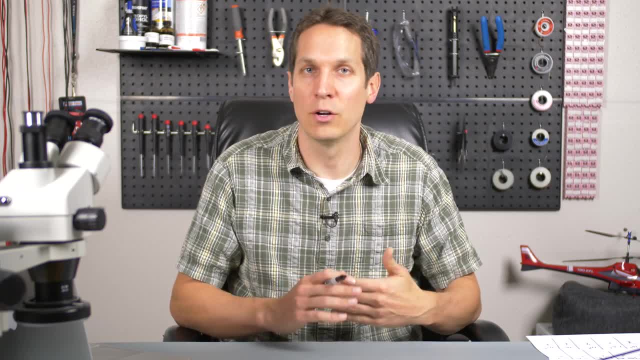 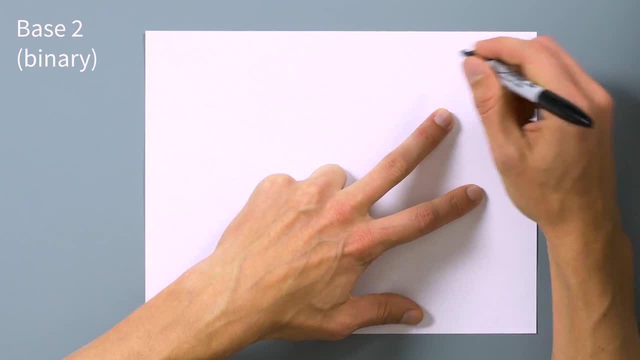 like that. It's always yes or no, And so that is why they use binary or base two. Now let's look at base two. So, instead of being 10 to the zero, 10 to the one, we have two to the zero, two to the. 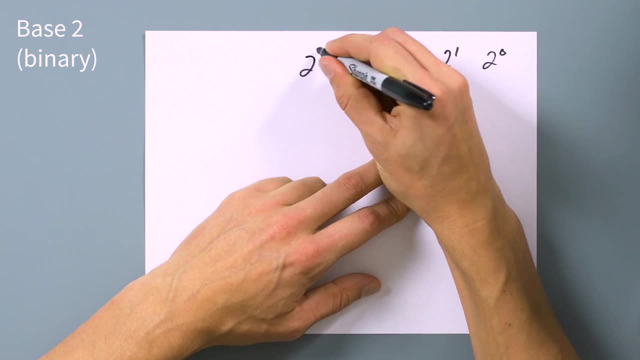 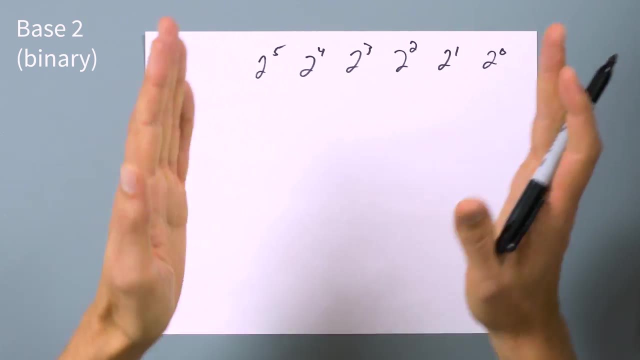 one, two to the two, two to three, Two to the four, two to the five, et cetera. And you have to go out farther because you can't get as many values in each slot. Instead of going from zero to nine, you can either say zero, one, 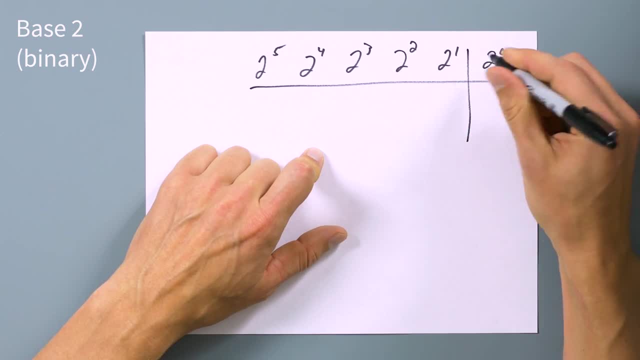 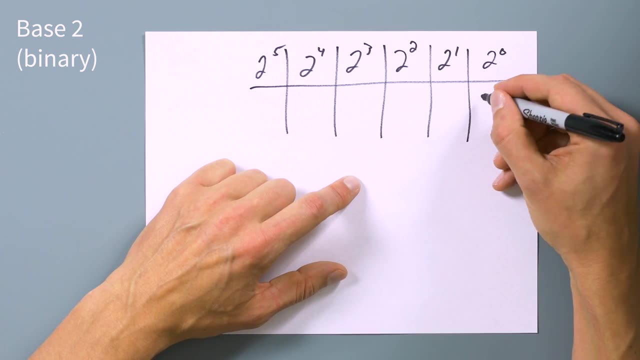 So these are multipliers, And then we can either choose that they are zero or one. So I am going to randomly put some numbers in here and I'm going to say one, one, zero, one, one. Now Two to the zero. 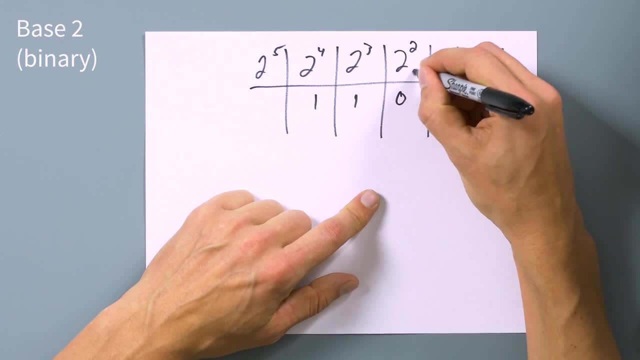 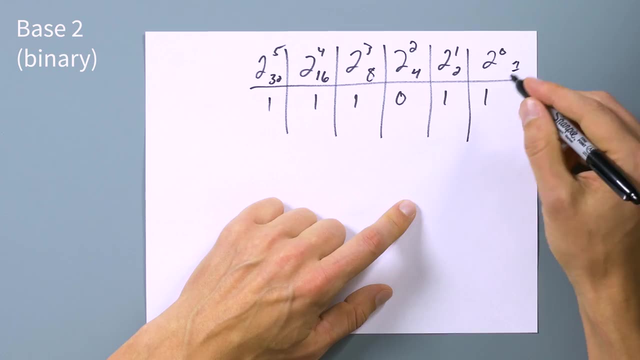 Is Basically one, Two to the one Is two, Two to the two, Four, Eight, Sixteen, Thirty-two- Let's just throw in another one there. Oh, that's going to be a big number. So now, if I want to look at this from a decimal- the way our brain works viewpoint- I can look. 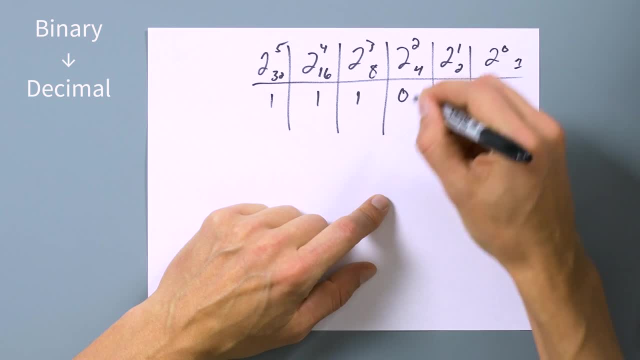 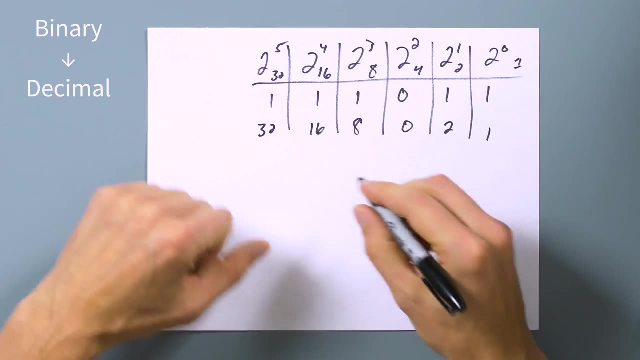 at this and say: one times one is one, One times two is two, Zero times four is zero, One times eight is eight, One times sixteen is sixteen, One times thirty-two is thirty-two, And then I can just simply add those together, which please don't make me do math in my head. 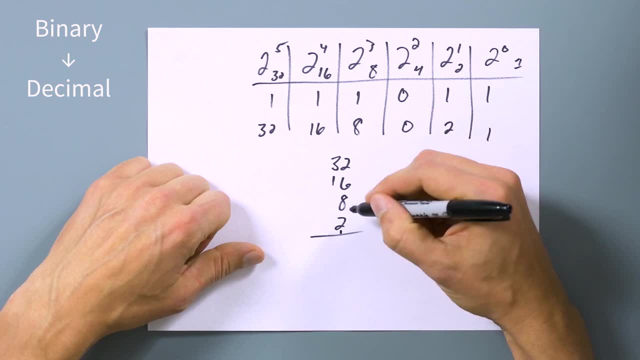 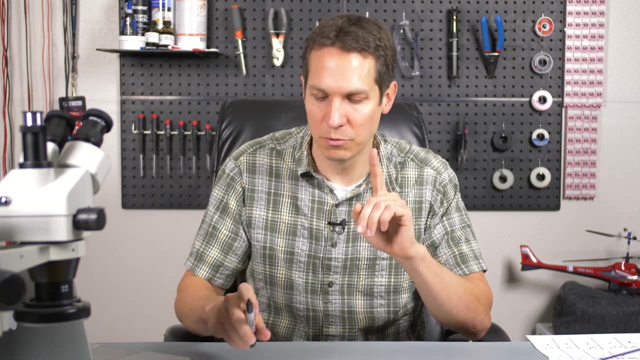 is: Oops, I forgot the one is going to be forty, fifty-six, fifty-eight, fifty-nine. Hopefully that is right. Let me pull up. I didn't pull this up before. I need to pull this up really quick. We actually have a binary to hexadecimal converter on Circuitbreadcom and I want to double check. 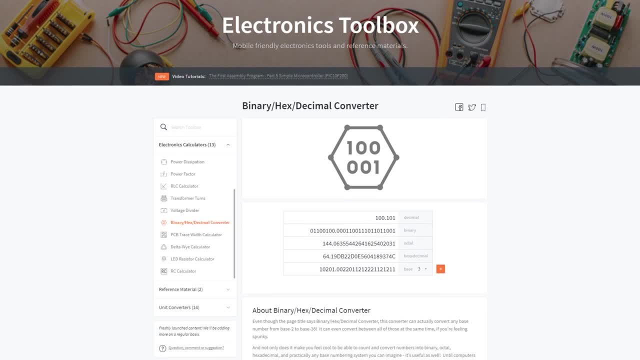 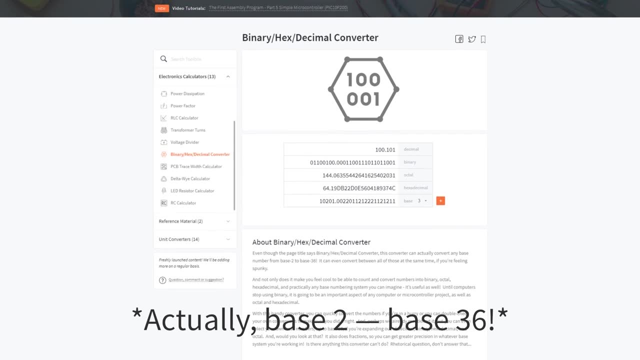 all my stuff before I make any assertions- And this is also down in the description, If you want to jump on here and check it out- it actually can convert anything from base two up to base twenty-six is, I think, how we set it up. 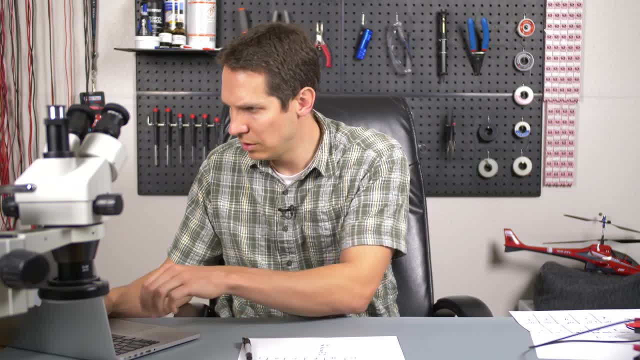 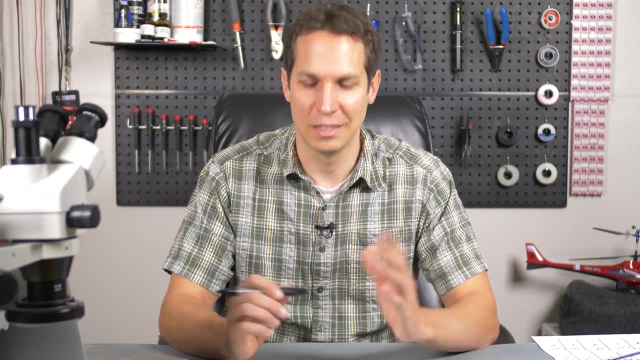 So let me one, one, one, One zero one one is fifty-nine. Okay, excellent, I did it right. It's something I feel pretty comfortable with it, but I do make a lot of arithmetic mistakes as well as I say the wrong words a lot, as you've probably noticed if you've watched. 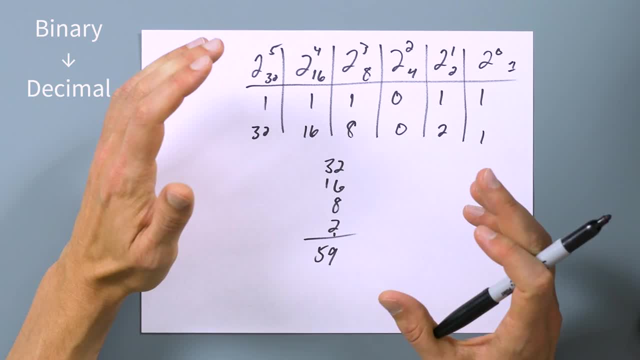 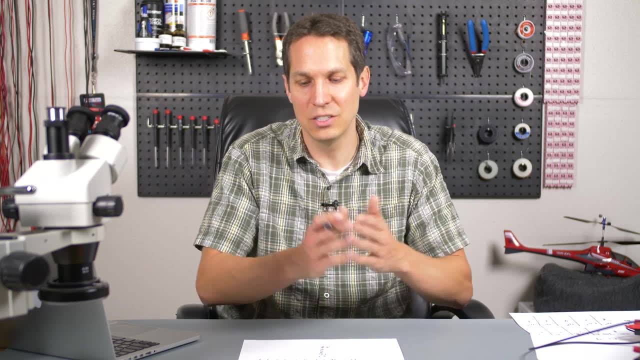 any of my videos. So this is the way that we can take a binary number and change it to a decimal number, and that's super helpful. But we also need to be able to take a decimal number and turn it into a binary number. Now I'm just going through paper like crazy here. 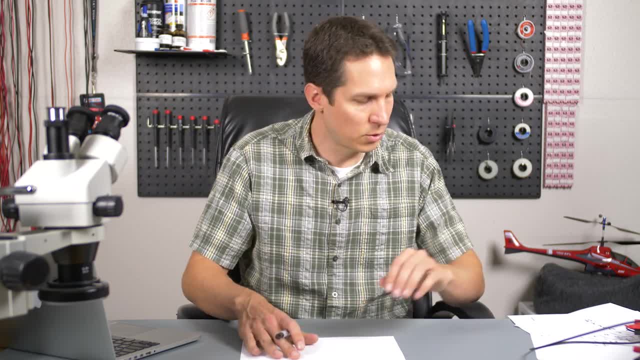 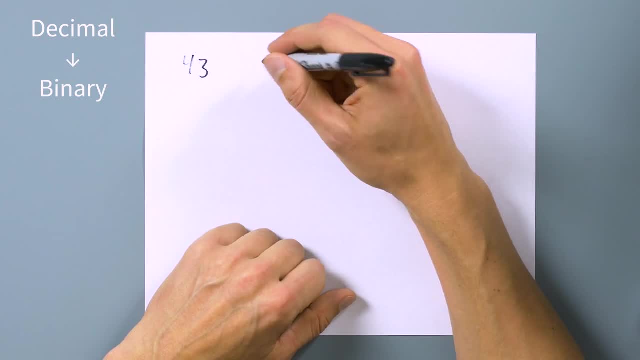 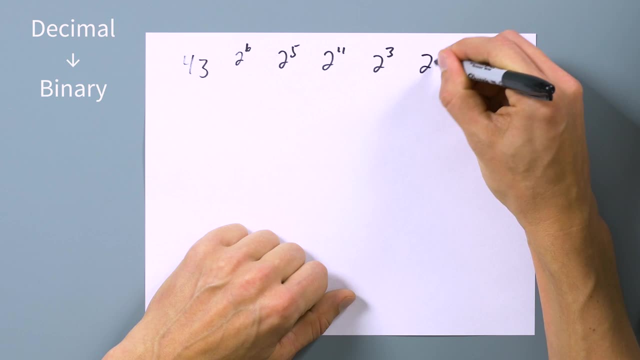 Let's go the opposite direction. I'm going to come up with a random number, So forty-three. Now we know that forty-three is less than sixty-four, So we know that it's going to be less than two to the six. So two to the five, two to the four, two to the three, two to the two, two to the one. 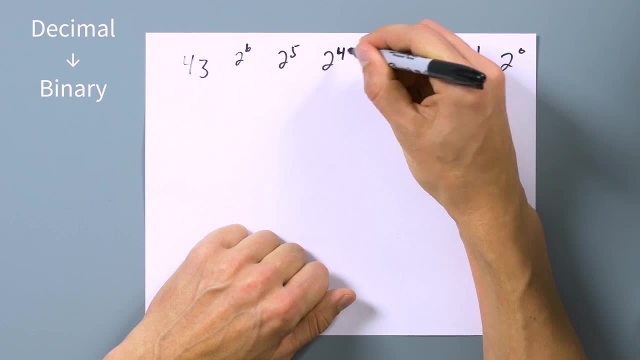 two to the zero, And if I haven't, I should apologize for my handwriting again. It is horrendous. So again, knowing this is sixty-four, thirty-two, et cetera, et cetera, So I'm going to do that. 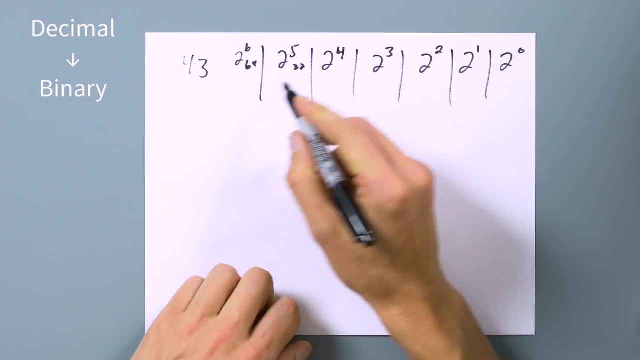 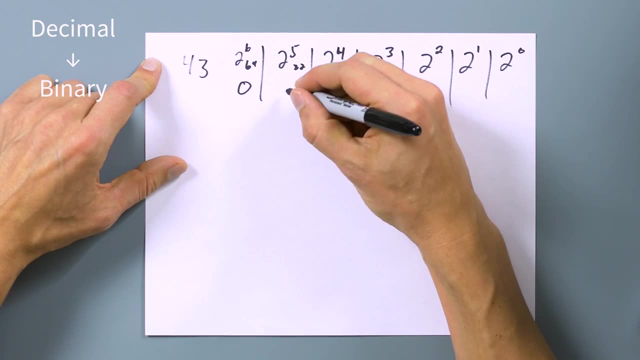 The way we go. the other direction is: you say, okay, forty-three, it's less than sixty-four, So I'm going to put a zero there. But forty-three is bigger than thirty-two, So I'm going to put a one there, and then I'm going to subtract thirty-two, which gives 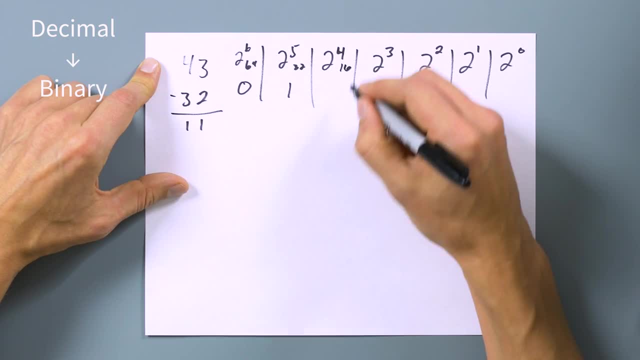 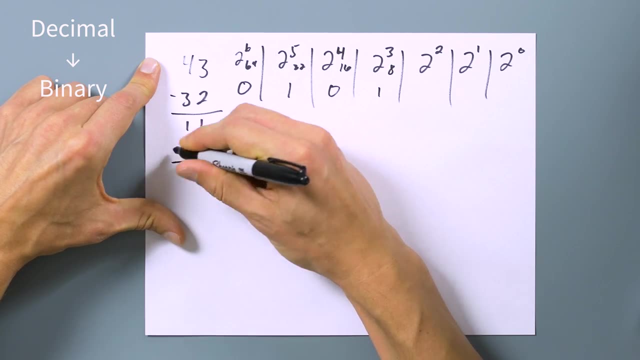 me eleven. Now I know that eleven is smaller than sixteen, So I'm going to put a zero there, but it's bigger than eight, So I'm going to put a one there. subtract it minus eight, gives you three, So two to the two is four, which is going to give me another zero. 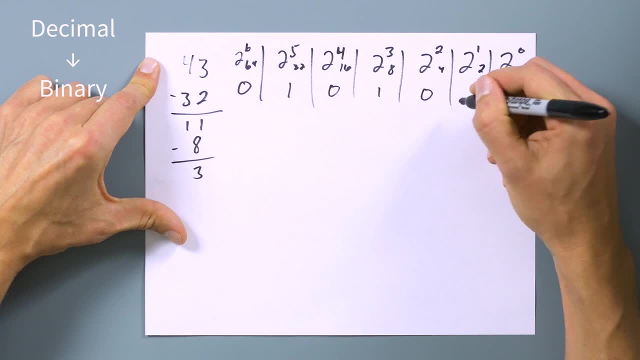 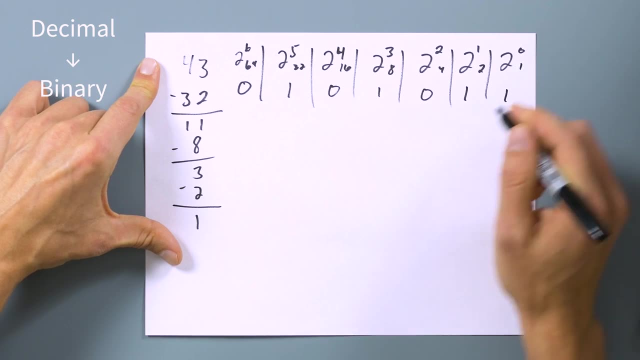 Two to the one is two, which gives me one minus two, and then two to the zero, which is one, is going to give me another one. So forty-three is zero one, zero one, zero one one. 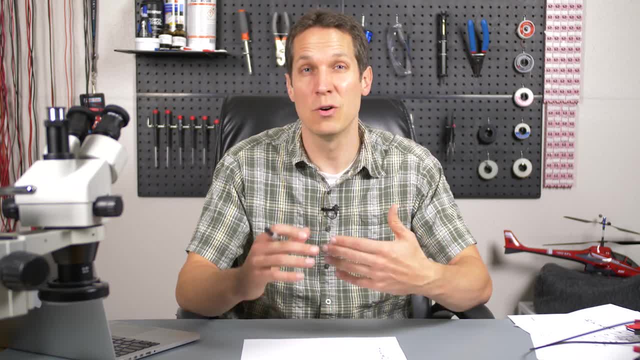 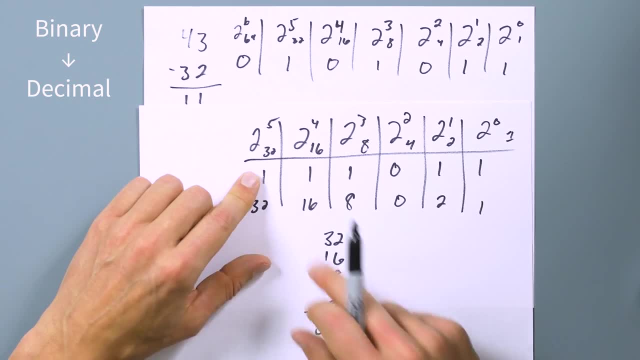 Now I would like to do a video later where we go through a couple more of these, because I know I'm going pretty fast, but right now I just want to focus on the concept. So when we were going from binary to decimal, we simply found out what each one of those 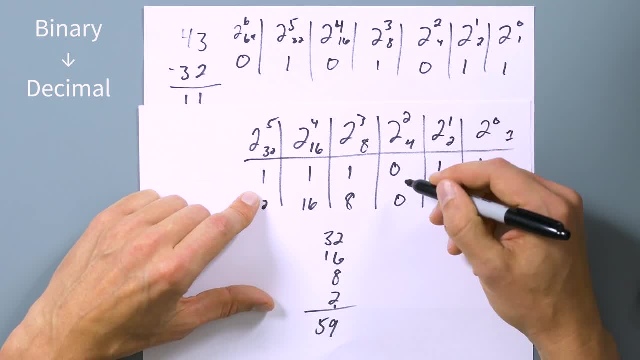 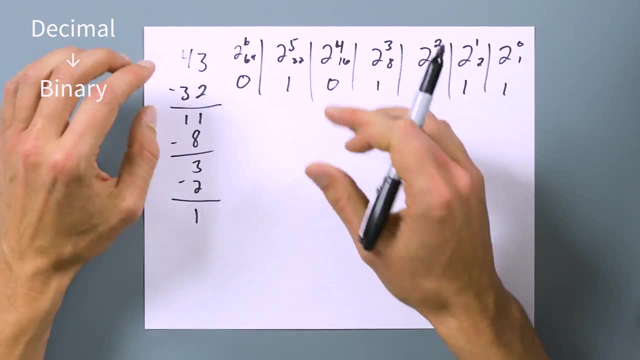 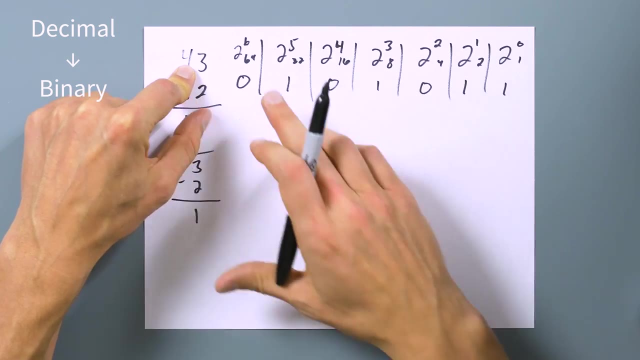 were and we added them together. So zero times four is zero and everything else. Just do some simple addition and then, going from decimal to binary, you have to do a little bit more intuitive thinking of. okay, that first number is: what is it smaller than? and 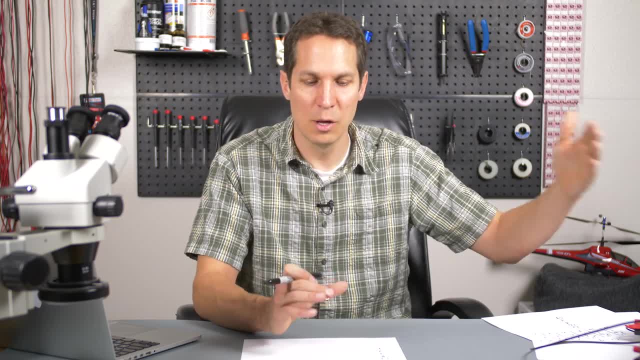 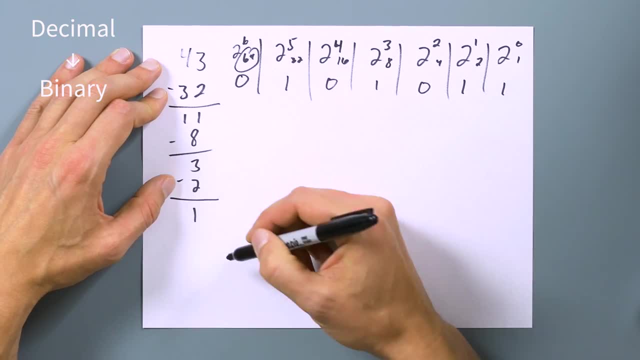 you'd have to know exactly where to start on your binary side. But once you figure out, okay, forty-three is less than sixty-four, I can start right there and then just go through down the line and subtract it. Now, this is very time intensive. 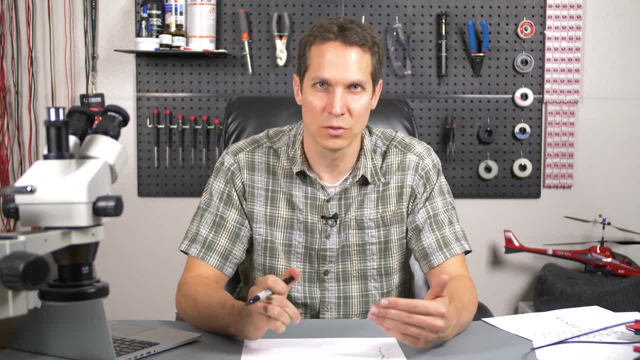 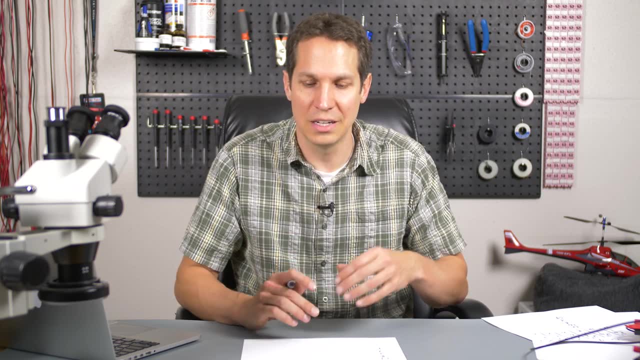 You'll never do this in real life. There's no reason for you to do this in real life. The only reason you should be doing this is to get a good understanding of what's going on, And once you have an intuitive understanding, one you'll be able to do some of the smaller 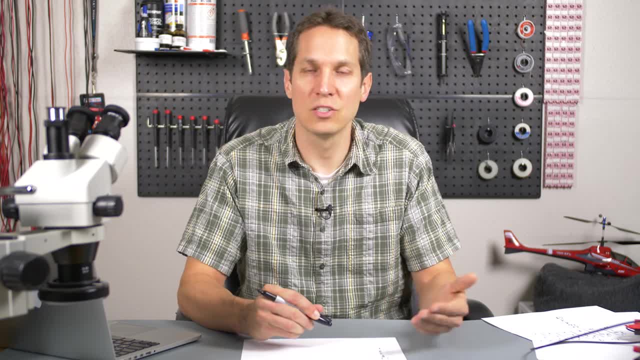 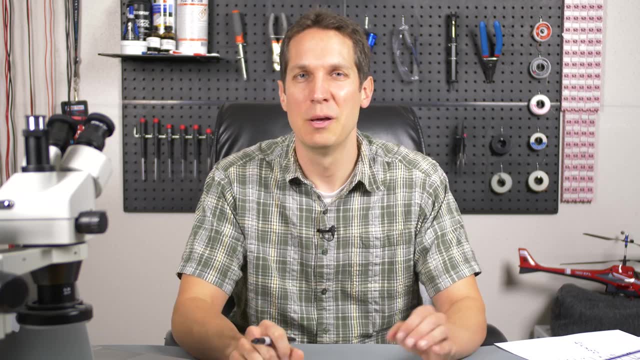 stuff in your head quite easily. and two, you'll be better prepared, so that when you go and use a converter, you type it in and you can do that quick. Does that make sense? Did I do that right? Yes, everything's great, but you're never going to be doing this in real life. 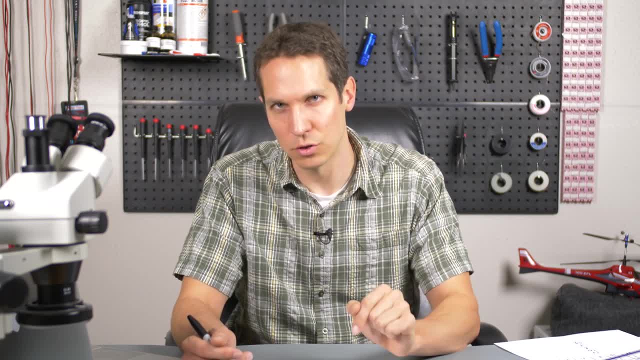 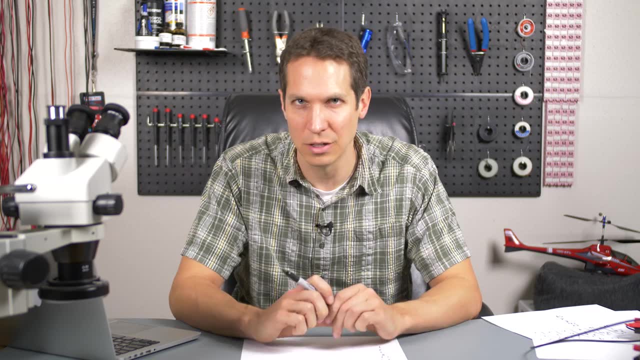 There's no reason, But understanding the concept. The concept is crucial. So now we've talked about decimal and binary and have gone from decimal to binary, binary to decimal. What is hexadecimal all about? Hexadecimal is beneficial because this is two to the six and you're getting seven digits. 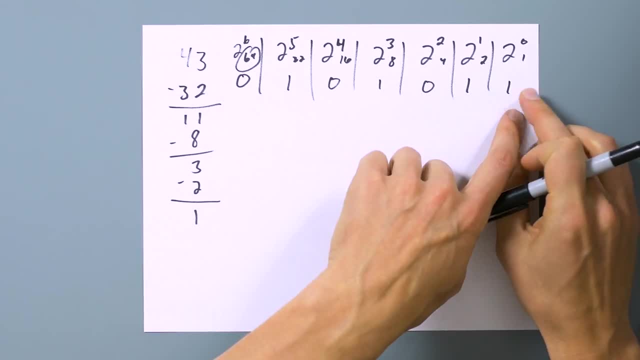 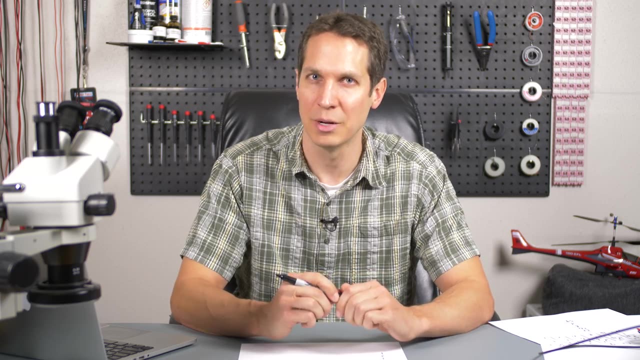 right there. Now we have sixty-four bit computers, which means that you have sixty-four ones and zeros, And I don't know about you, but I can't keep that many ones and zeros straight in my head. Honestly, even with hexadecimal it's still difficult. 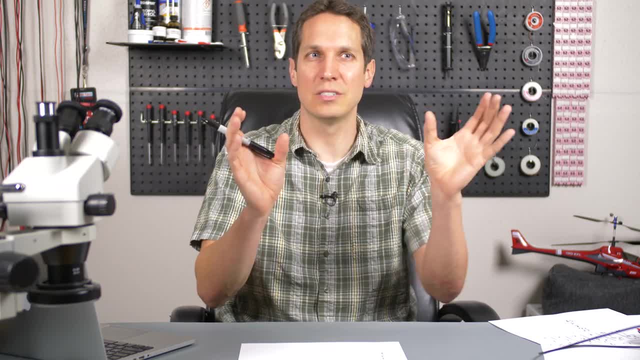 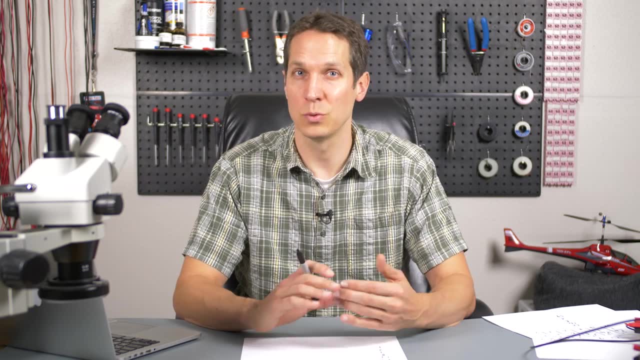 But what hexadecimal does Is it simplifies things and it makes what seems like a bunch of just random ones and zeros into something that's a little bit more human, readable And, because of that, a lot of compilers when you're doing embedded systems, like with microchip. 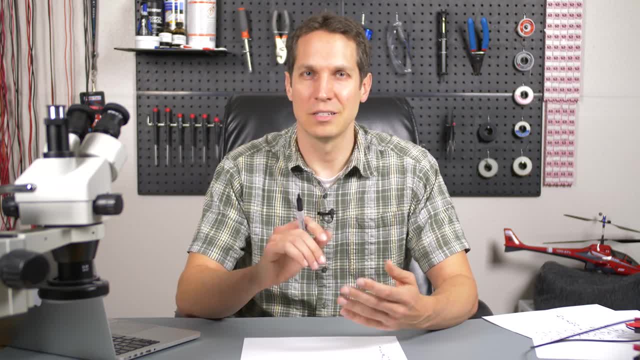 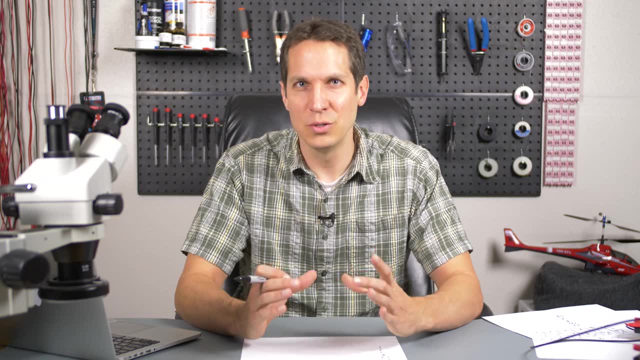 at now. now they're the same, I guess renaissance. well, I don't know why. I'm listing all of these STM, NXP, whatever Most of them do, their IDEs, so that it naturally the number you put in is hexadecimal versus. 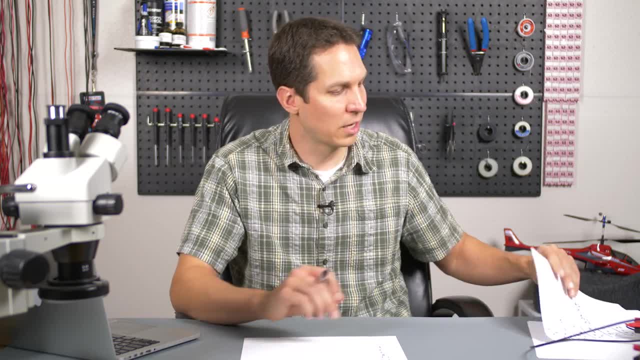 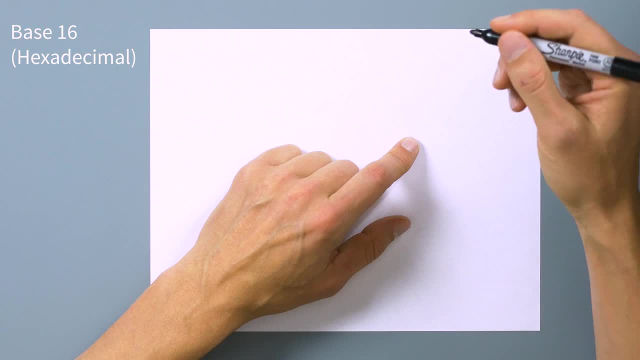 decimal, which can really screw you up. So let's go over hexadecimal really quick. Hexadecimal is base 16.. So we were doing 10 to the zero, 10 to the one, and then two to the zero, two to the one. 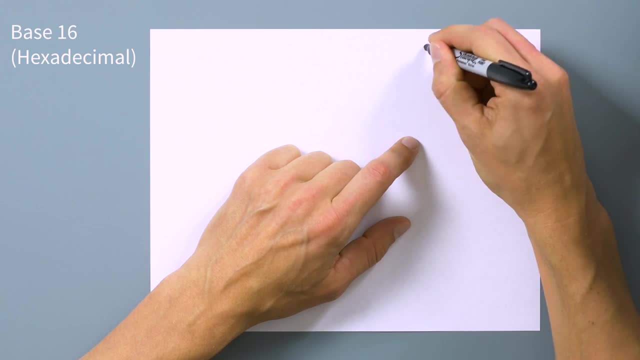 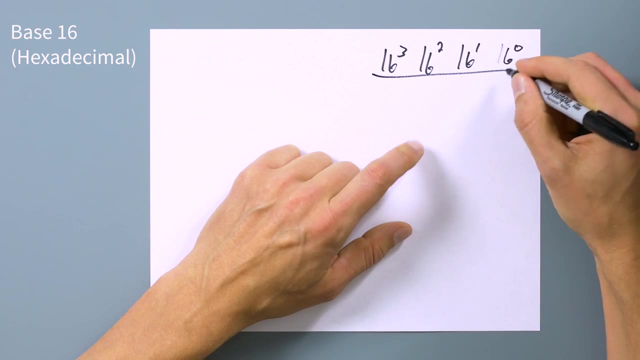 Now we're doing 16,: 16 to the zero, 16 to the one, 16 to two, 16 to three, And frankly I can't do this sort of math in my head. So that comes out to be zero to 16.. 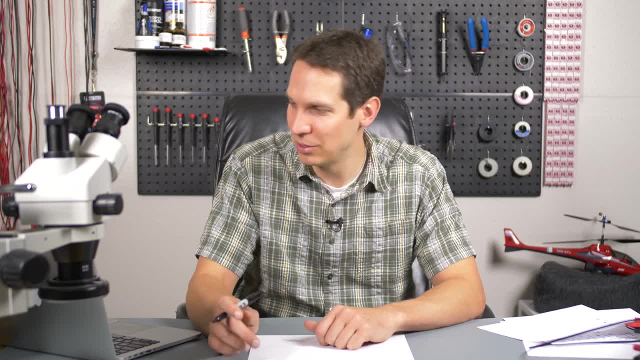 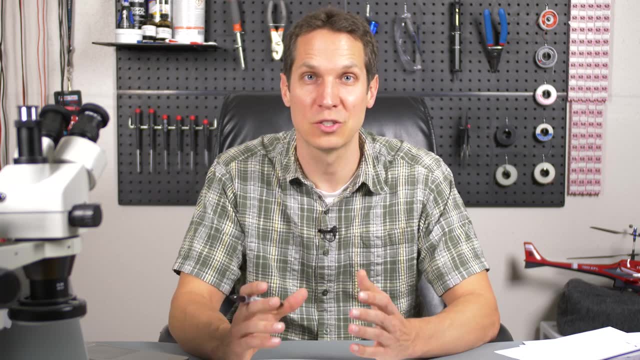 And then this is: Wow. Okay, I'm really thrilled I got myself off here. I have to admit that hexadecimal is harder for me to do in this, because the numbers are so much bigger and I can no longer do the math in my head. 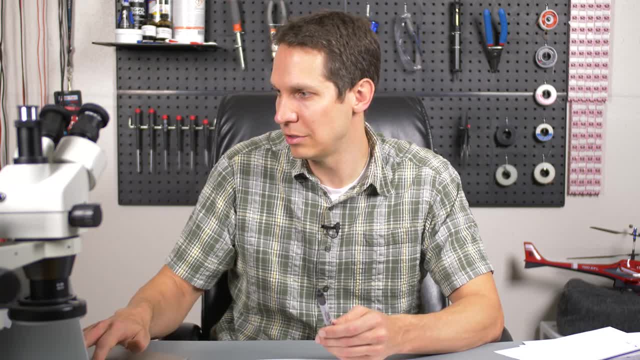 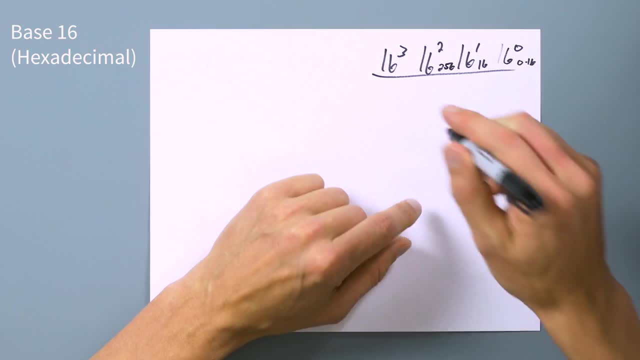 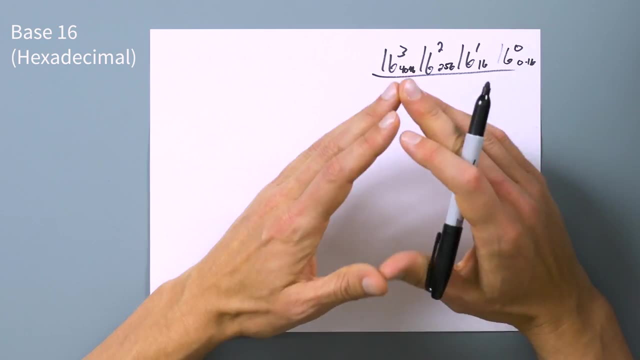 So I'm going to do some quick cheating: 16 times 16 is 256- I should have known that. and then do another 16 in, there is 4096.. So you can see this gets big very, very, very fast And the basic concept is the same. 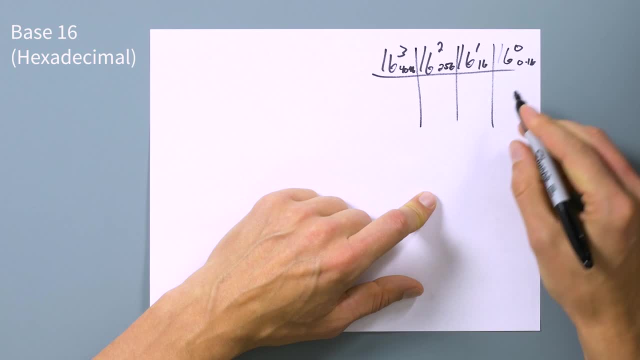 That whatever is in Each of these slots is then multiplied by whatever is up here, which in this case is one. This case is 16 256 4096.. Now the challenge here is that, like I said before, I called 10 the what would come after. 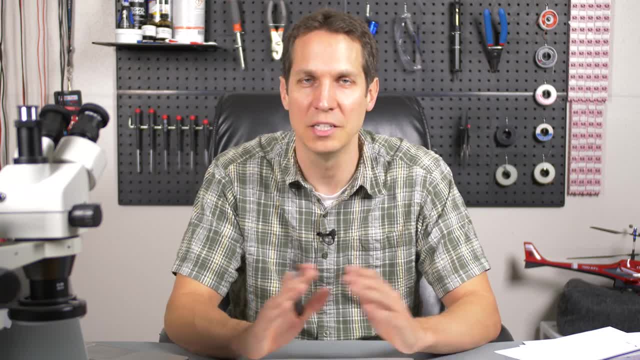 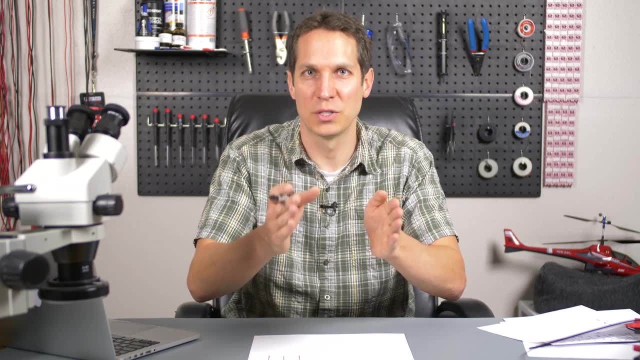 nine. I called it Bob just because that's kind of a random name. I give anything, But in reality we need actual numbers to represent 10,, 11,, 12,, 13, and 14.. Because, again, it's zero to 15.. To give us our 16 digits Now, because most of us know the ABCs. they just decided that would be a very simple way to represent the additional numbers. So instead of zero to nine, it's zero to F: 0123456789,, ABCDEF and F is equivalent. 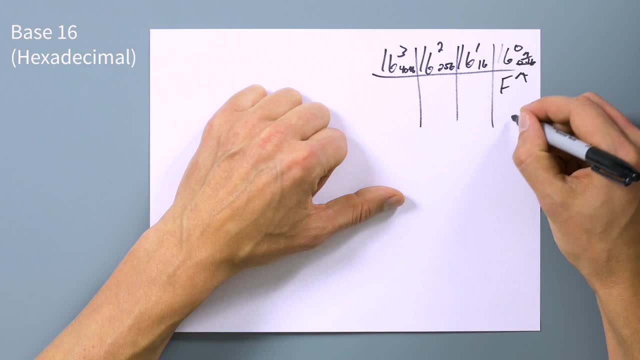 to 15.. So if I put F here, that's F times one, and so that's 15 times one, which equals 15.. But then if I put over here 16, if I put F, that's F times 15.. 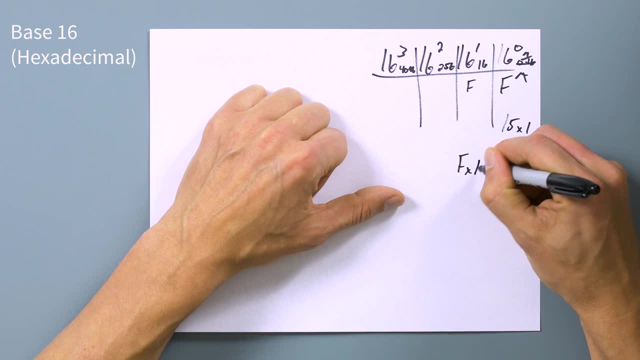 So that's 15 times one, which equals 15.. But then if I put over here 16, if I put F, that's F times 15.. So that's F times 16, which is going to be 16 less than 256.. 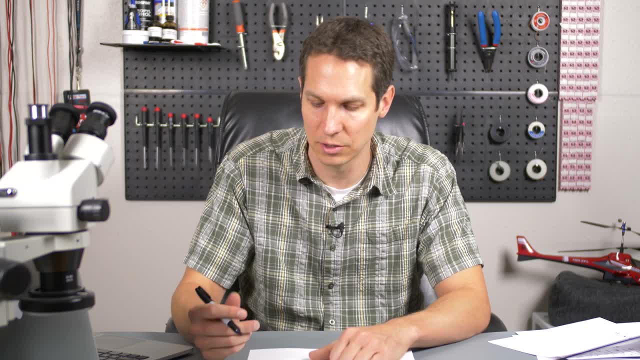 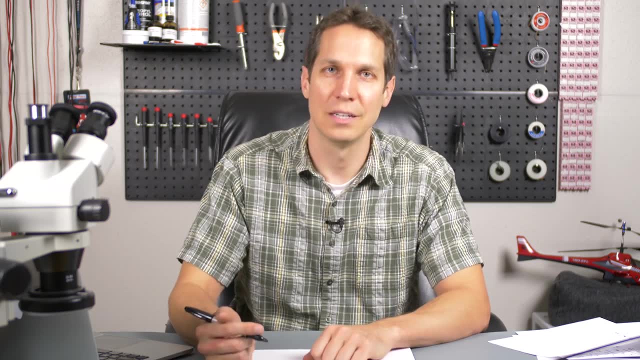 So what is that 240?? Oh, I really hate doing math on camera. I get very self conscious and certain that I'm going to destroy things. So, 15 times 16, 240- Yes, actually, one of the biggest challenges here is when you don't. 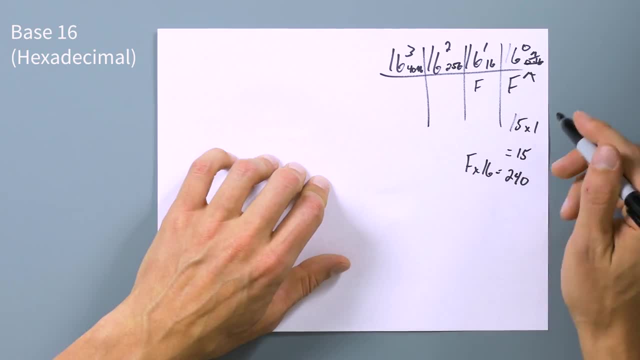 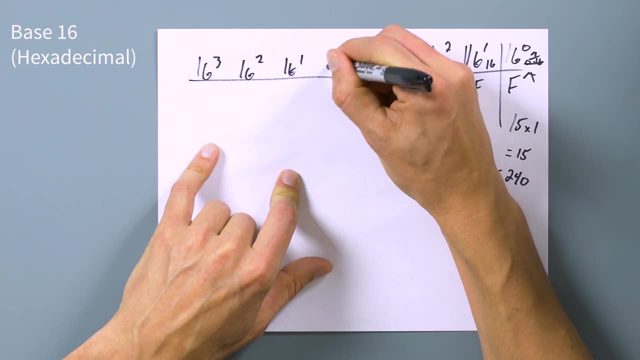 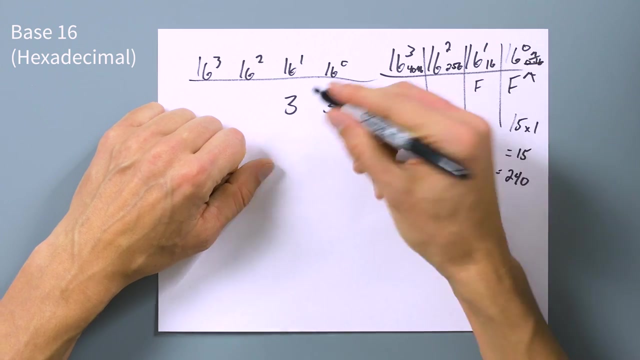 see Fs. when you don't see the letters, that's when people screw up. So sometimes you'll see something where you're doing your numbers and you'll see somebody. see, see somebody, right, 3333,, right there, so you. 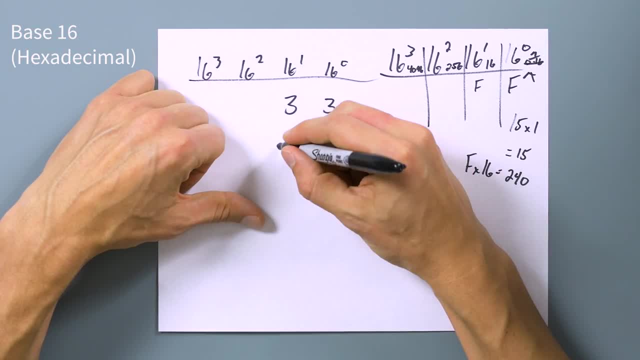 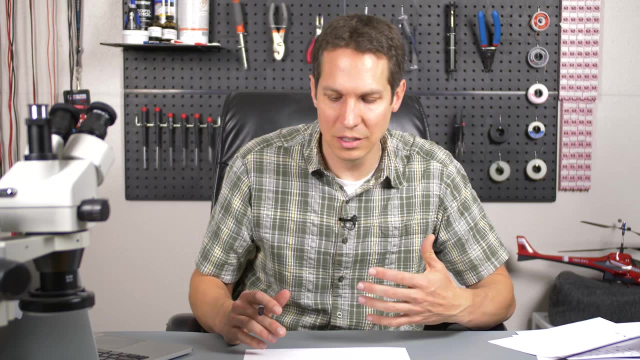 think, oh, 33.. Sweet, I know that that's 33. But in reality that's three times 16, plus three, which is a vastly different number than 33.. So one of the things that they do to make it easier and, unfortunately, sometimes it. 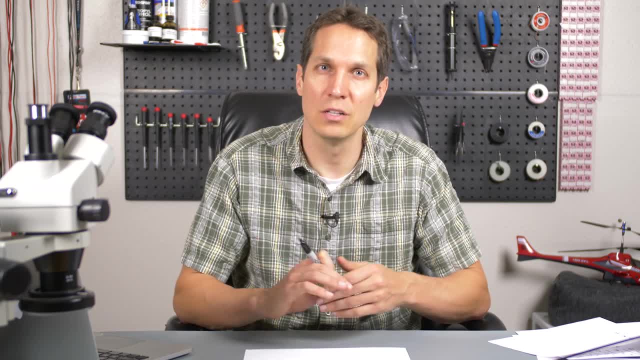 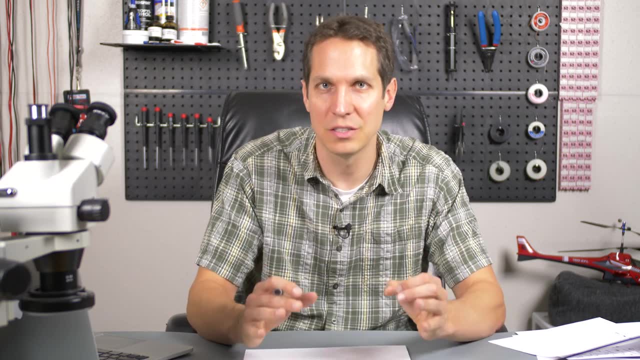 just defaults to hexadecimal, which is again what happens in a lot of the IDEs out there. But if you want to, you can do that. If you say no, I want this to be decimal or binary, or explicitly state that it's hexadecimal. 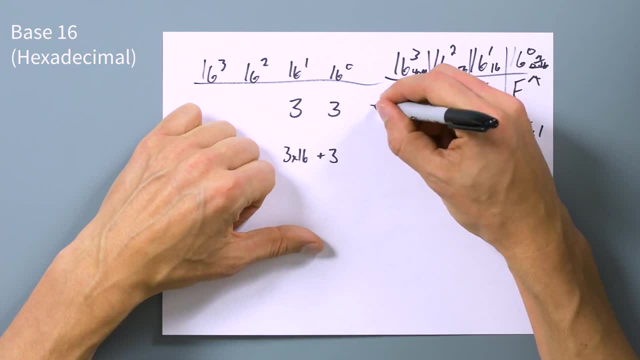 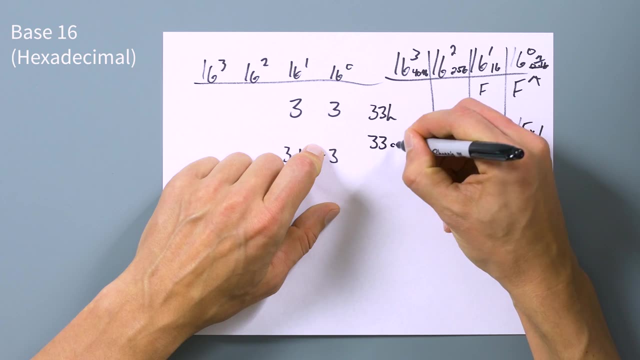 you usually put an H, B or D, depending on what you have. So for here you'd have 33, H to show that that's 33 hexadecimal. Now if you wanted that to be decimal, you'd do 33, D and then binary. you can't do 33.. 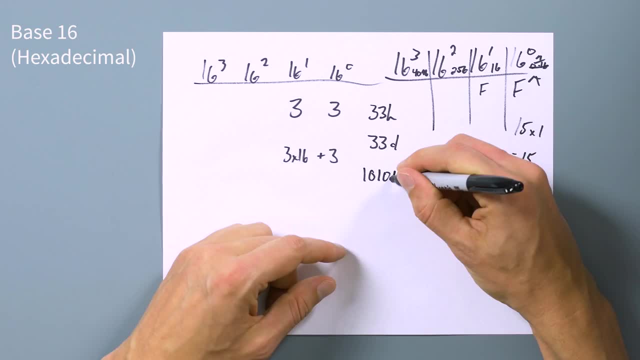 But you'd at least have 1010, B, to make sure people don't think that's 1010.. Now you'll also see hexadecimal written out as 0x1010.. So if you want that to be decimal, you'd do 0x1010. 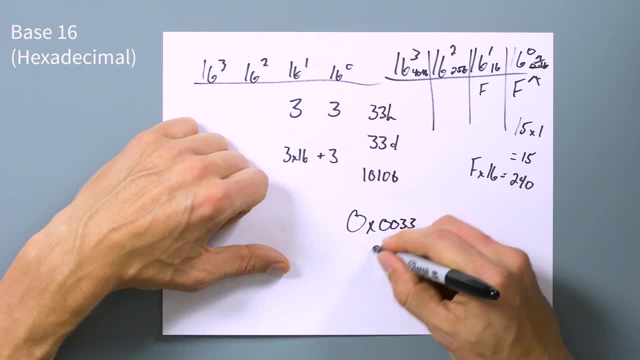 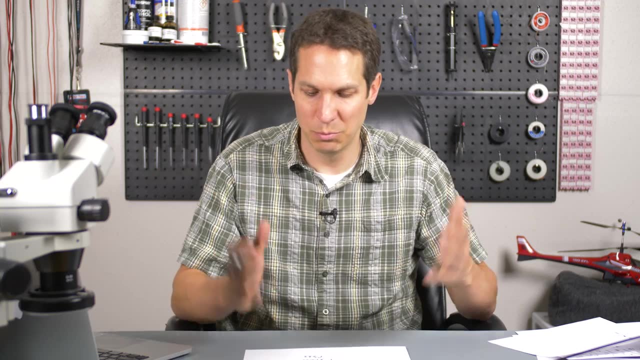 If you want that to be hexadecimal, you'd do 0x0033, or just 0x33.. So 0x or 33, H, that's two different ways of showing hexadecimal, But both of them work and you'll see them so much that once you see this, you'll see 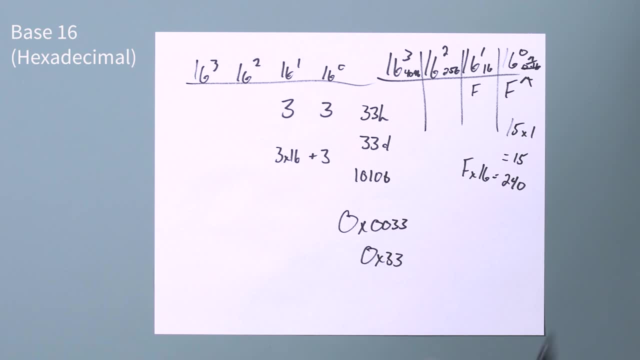 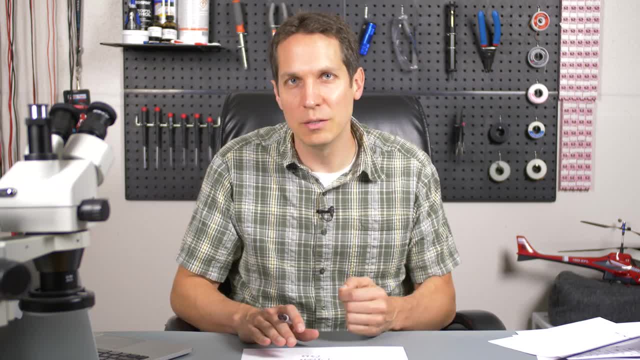 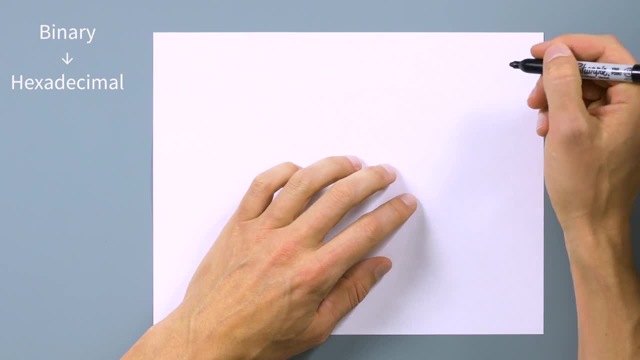 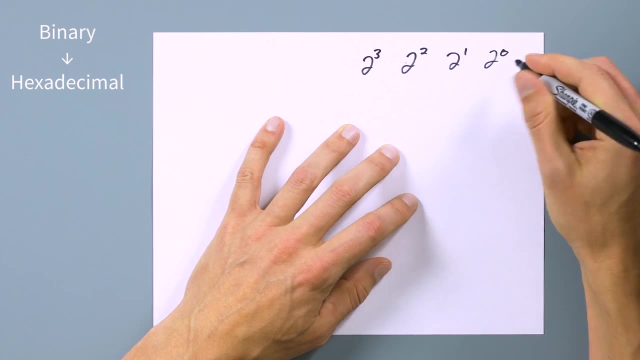 You typically do your conversions between hexadecimal and binary, which is incredibly easy, So let me grab another piece of paper. So one of the beautiful things about binary and hexadecimal is binary: you go 2 to the 0,, 2 to the 1,, 2 to the 2,, 2 to the 3, and that gives you 8,, 4,, 2,, 1 as your multipliers. 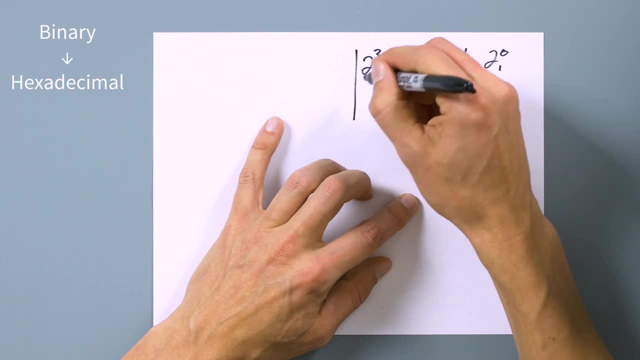 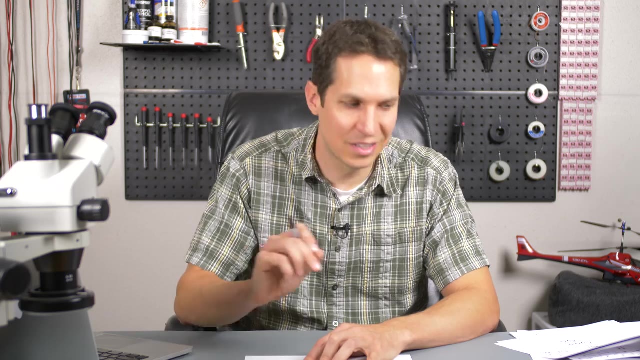 8,, 4,, 2, 1 as your multipliers. 8, 4, 2, 1 as your multipliers. And so this range, And so this range, This subset right here can give you any value between 0 and 15, which is exactly what one. 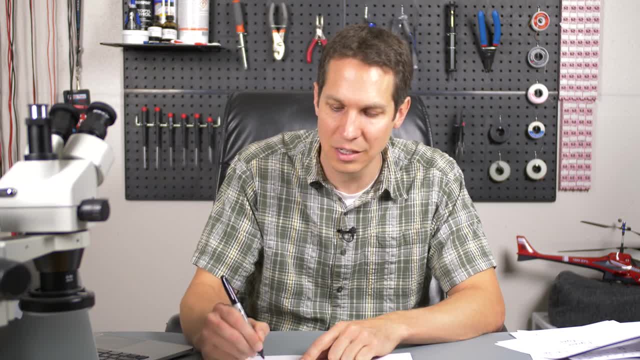 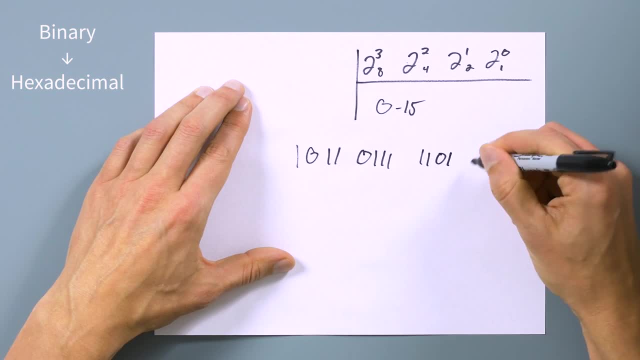 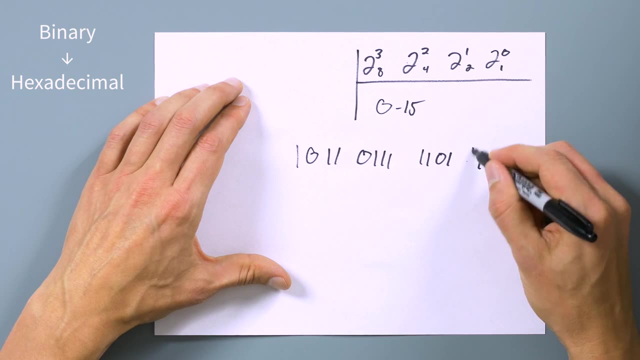 character in hexadecimal can do So. the way this is so easy is that, instead of I'm just going to write a bunch of random ones and zeros- and Hopefully those are super random- And notice how I gave them a little space between each one, because now I can take each one. 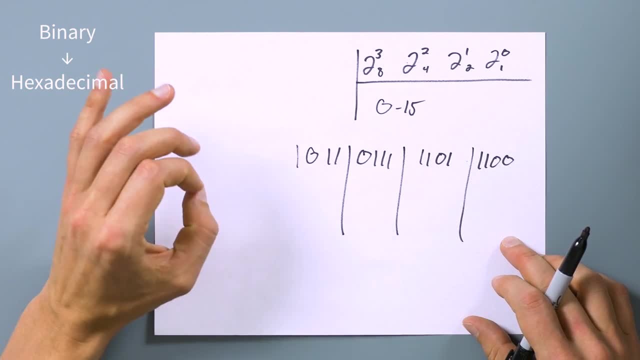 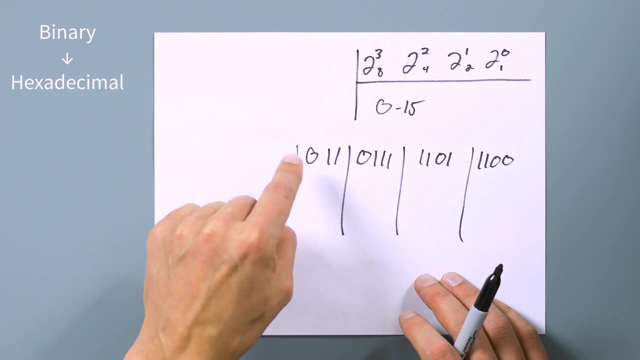 of these and turn it into very random, Beautiful, Perfect, Perfect them into a very simple hexadecimal value that is then very easily shown, And so, instead of having to remember 0110, excuse me, 10110111111011100,, I can look at this converted to. 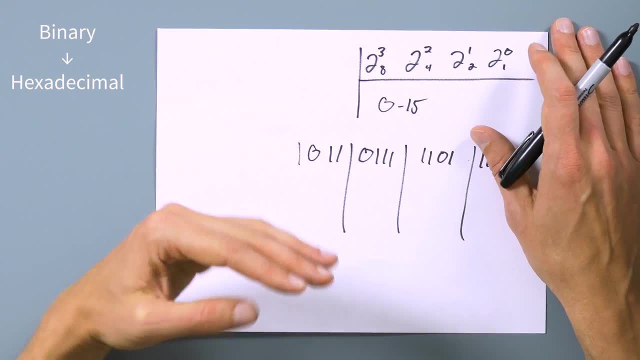 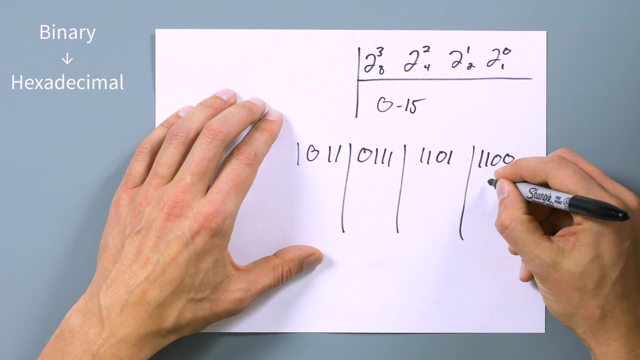 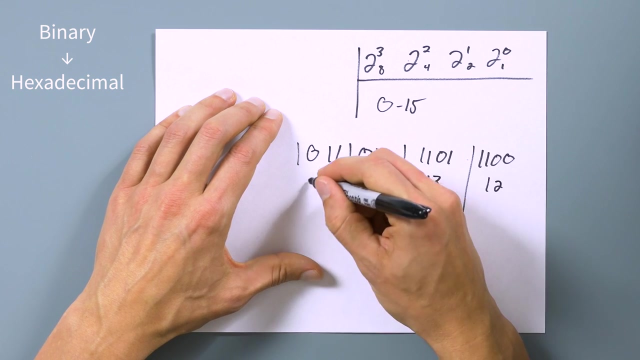 hexadecimal, and then I only have to remember four. much easier to remember numbers. So give me a second. I'm going to calculate these out, hopefully not embarrass myself too bad. This looks like it's 12,, which would make this 13,, which make this seven, which makes this 11.. So in hexadecimal, 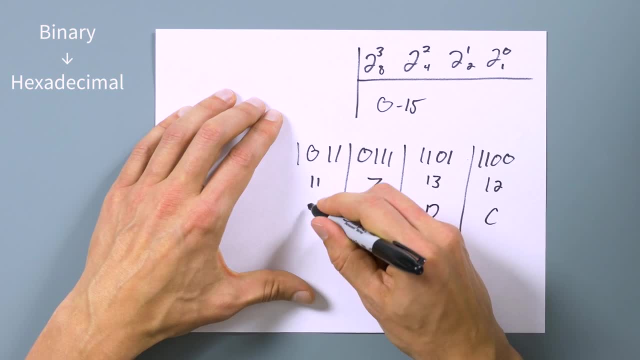 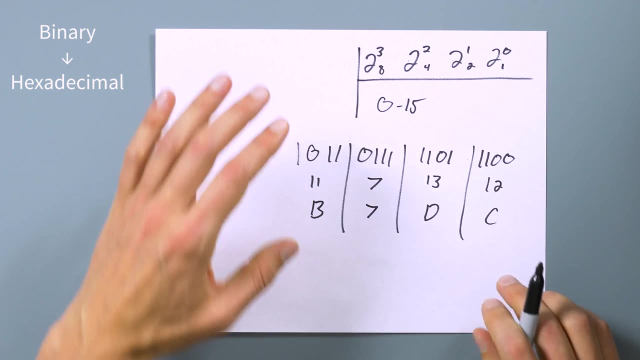 this would be ABC, D, B seven, So I could write all of this crazy stuff which I am already going to forget, And then I can just look at this B7, DC. it sticks with your mind so much better.